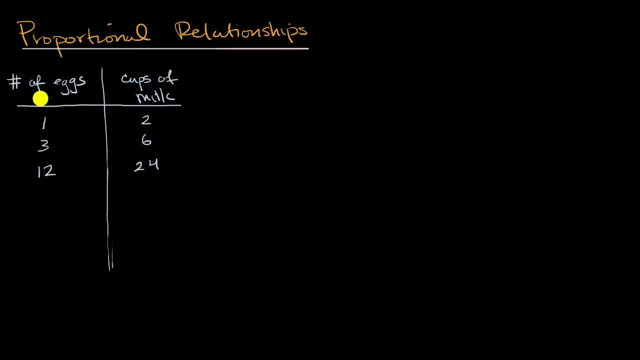 and the number of eggs. Well, to test that, we just have to think about the ratio between these two variables And you could say the ratio of the number of eggs to cups of milk or the ratio of the cups of milk to the number of eggs. but just to ensure, 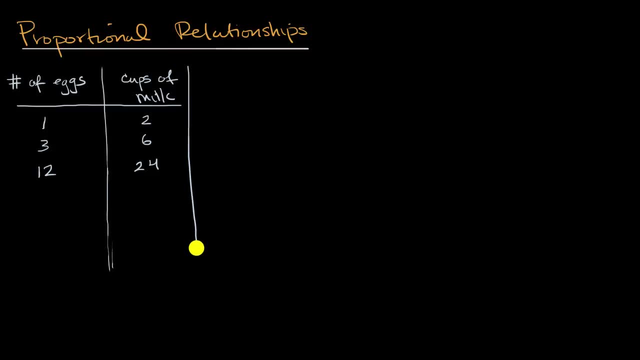 that they are always equivalent in these scenarios. So let me make another column here, And I'm going to think about the ratio of the eggs to the cups of milk. Well, in this first scenario, one egg for two cups of milk. The second scenario is three to six. 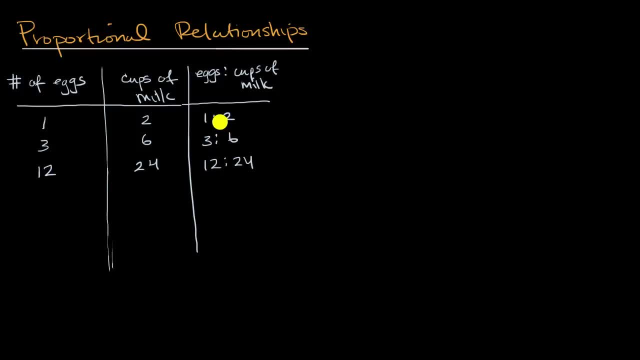 This third scenario is 12 to 24.. Are these equivalent ratios? Well, to go from one to three, you multiply by three. And we also, to go from two to six, you multiply by three. So you multiplied both the variables by three. 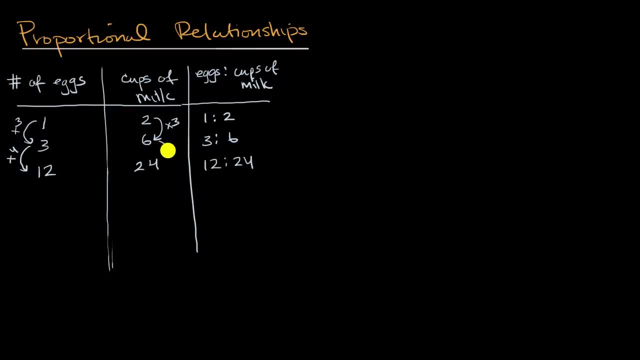 Similarly, if you multiply the number of eggs by four, then you multiply the number of cups of milk by four as well. So these, indeed, are all equivalent ratios: One to two, three to six, 12 to 24.. In every scenario, you have twice as much cups of milk. 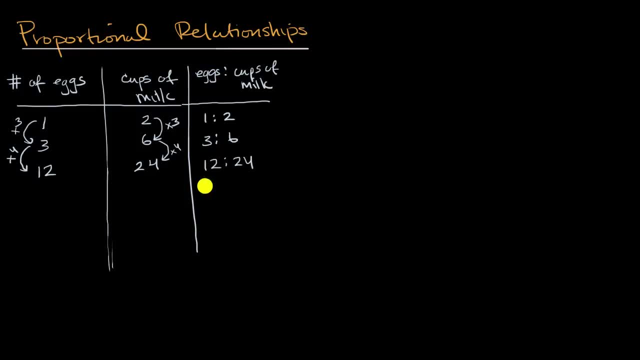 as you have number of eggs, So this would be proportional. So check Now what would be an example of a non-proportional relationship. Well, let's stay in this baked goods frame of mind. Let's say you're going to a cake store. 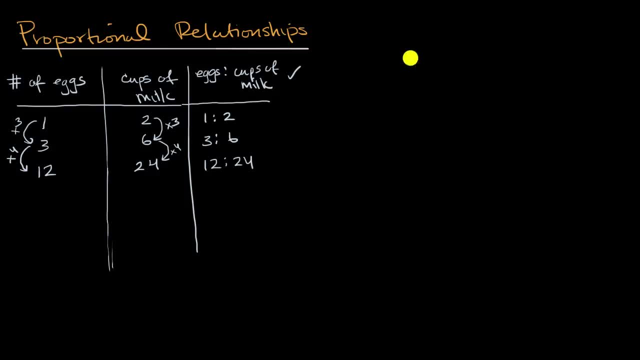 and you're curious about how much it would cost to buy cake for different numbers of people. So let's say numbers of servings, number of servings in one column and then the cost of the cake, And let me set up two columns right over here. 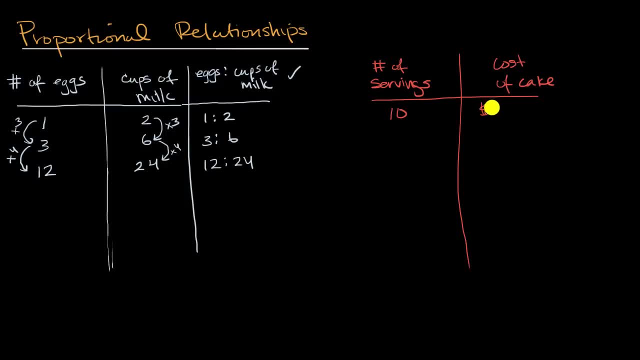 And so let's say, if you have 10 servings, the cake costs $20.. If you have 20 servings, the cake costs $30.. And if you have 40 servings, the cake costs $40.. Pause this video and you see if you can figure this out. 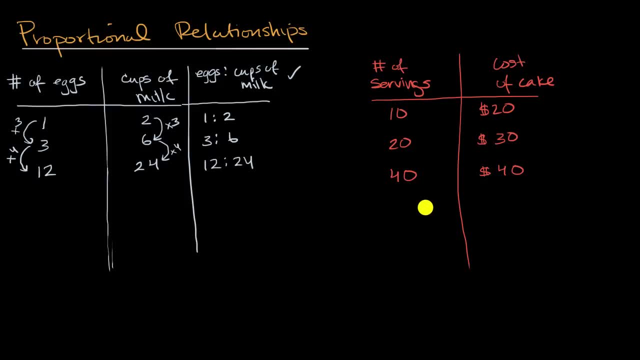 Pause this video and you see if you can figure this out. Pause this video and you see if you can figure this out, Whether this is a proportional relationship. If it is, why? If it isn't, why not? 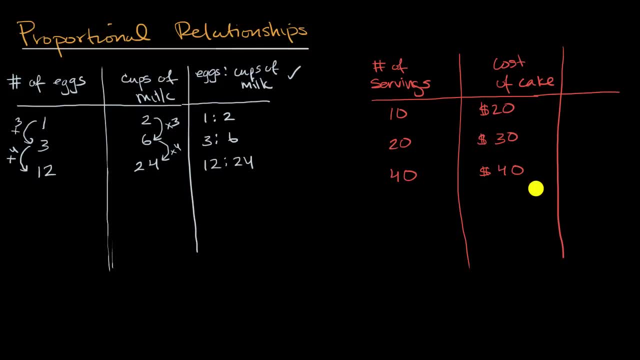 All right. well, let's just think about the ratios again. So- and here are two variables- are the number of servings and the cost of cake. So if we look at the ratio of the servings, servings to cost, So in this first situation it is 10 to 20,. 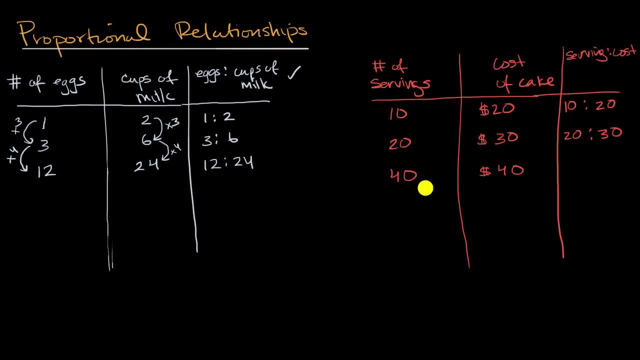 and then it is 20 to 30, and then it is 40 to 40.. And so to see if these are equivalent ratios, when we go from 10 to 20 on the number of servings, we're multiplying by two. 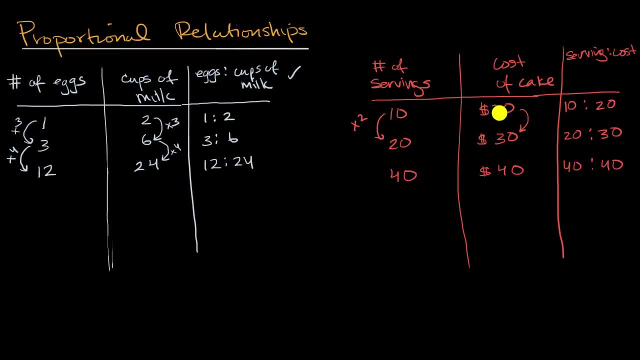 But when we go from 20 to 30 on the cost of the cake, we aren't multiplying by two, we're multiplying by 1.5, or one and a half. And similarly when we go from 20 to 40,. 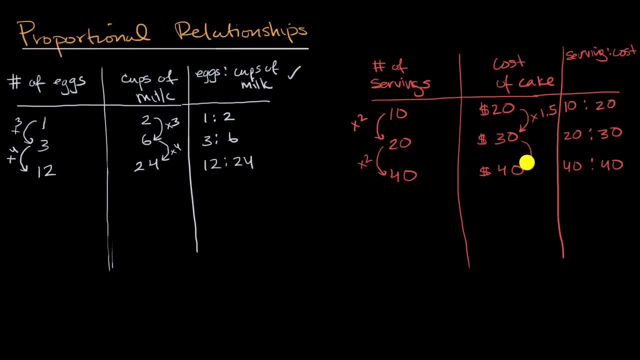 we are multiplying by two again, But to go from 30 to 40, we aren't multiplying by two, we're multiplying by one and one third. By one and one third, When we multiply our servings by a given amount, we're not multiplying our cost of cake by the same amount. 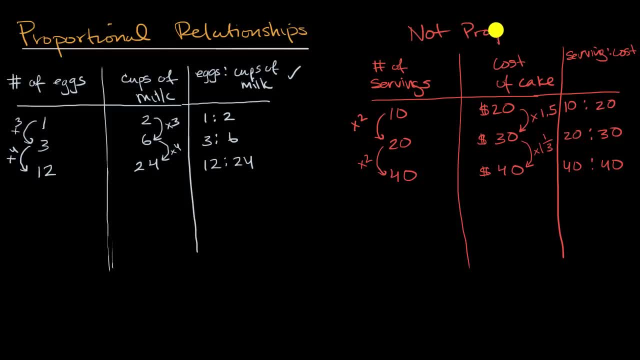 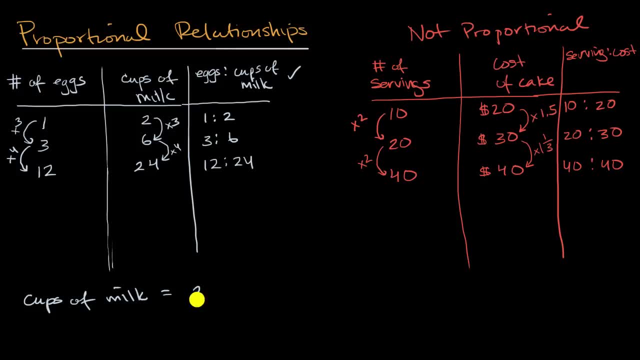 So in our first example right over here, we said: the cups of milk is always constant times the first. So in our first example right over here, we said: the cups of milk is always constant times the first, always going to be equal to two times the number of eggs. 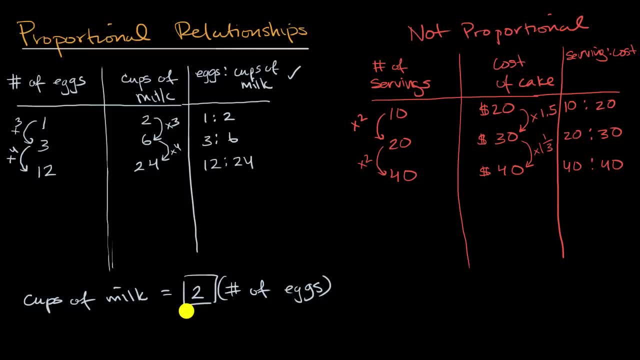 And this number right over here. we call that the constant of proportionality, And you wouldn't be able to set up an equation like this in this scenario. It would have to be more complicated. And so a proportional relationship. the ratios are equivalent between the two variables.